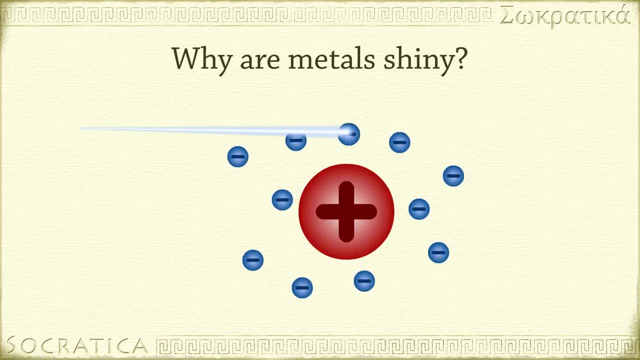 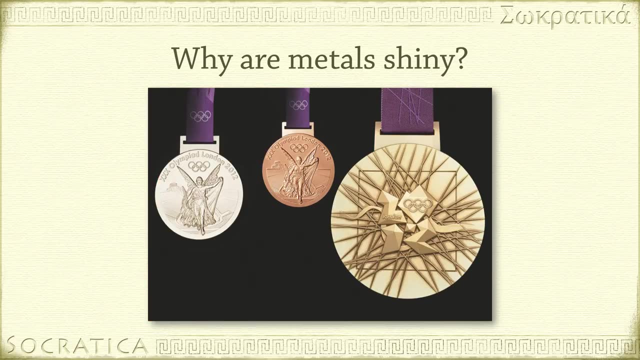 The. when they fall back down a level, the energy is re-emitted as light. The color of the metal is determined by the wavelength of light which is re-emitted. Similarly, this free flow of electrons explains the ability of electrons to absolutely fence. 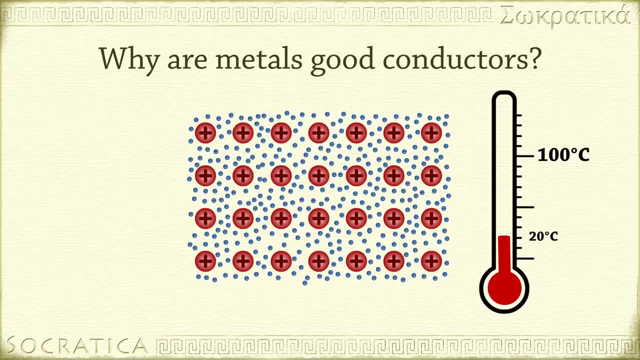 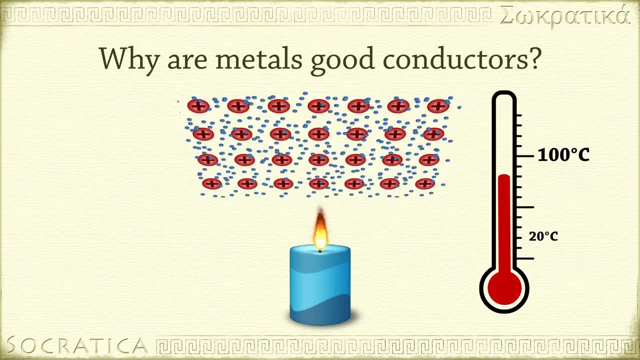 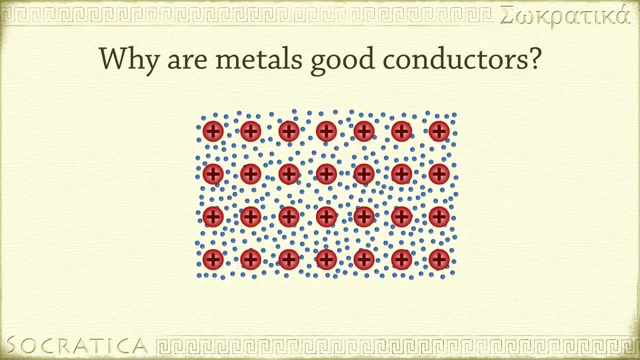 the moving losam ability of metals to conduct heat and electricity. When you heat up a metal, the free electrons quickly start vibrating. Increased kinetic energy means increased temperature. When an electric current is applied to a metal, electrons enter from one side, causing repulsion and 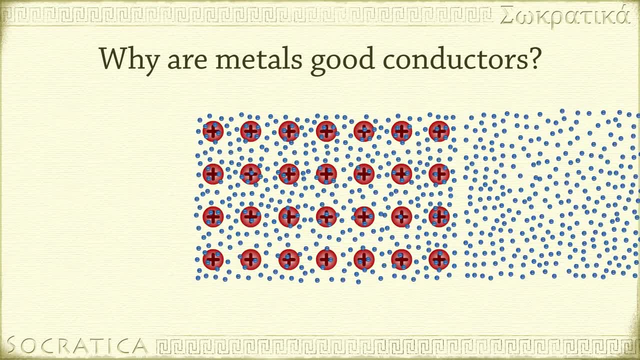 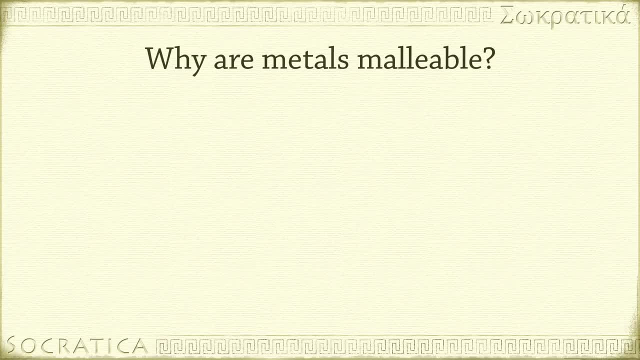 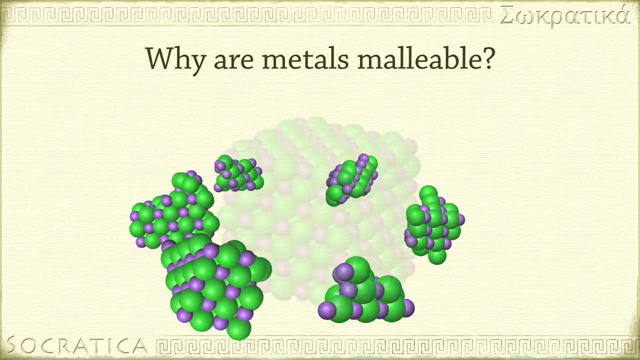 generating movement within the sea of electrons, and an equal number of electrons exit the metal, as the number that entered The mobile sea of electrons also explains the malleable nature of metals. If you strike an ionic crystal with a hammer, it shatters. This is because the applied force pushes like 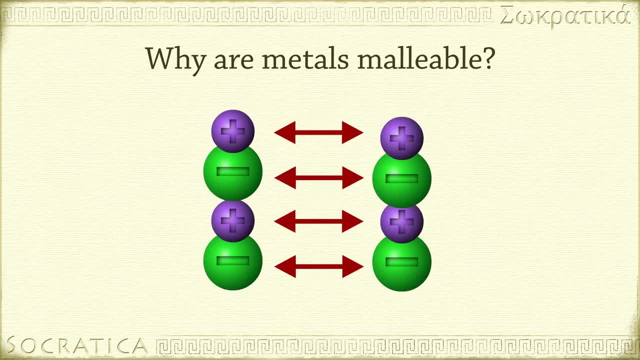 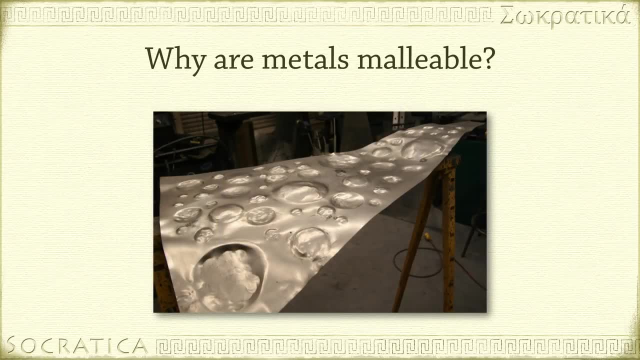 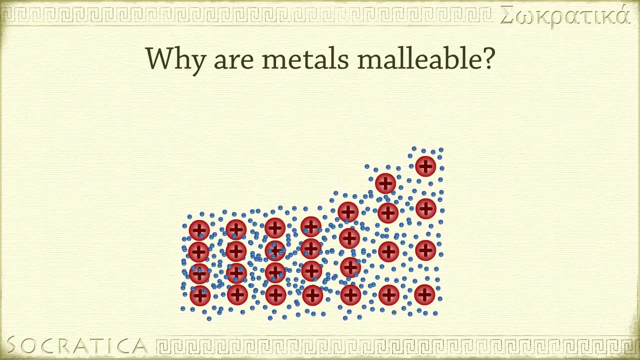 ions close together, They violently repel each other, breaking the crystal apart. In contrast, if you hit a metal with a hammer, it doesn't break, It just dents. Metals are able to deform in response to an applied force. The mobile sea of electrons also explains the malleable nature of metals. If you strike. 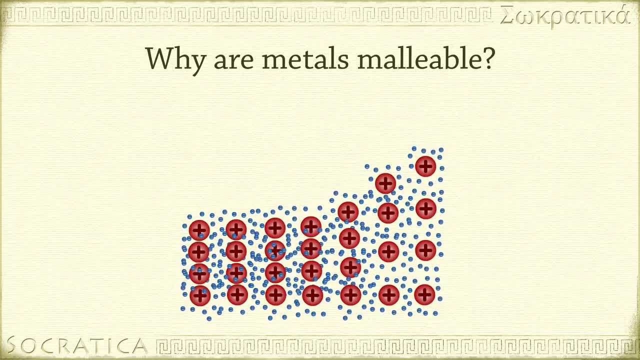 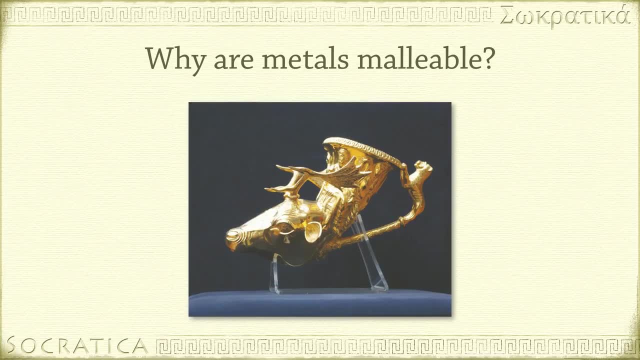 an ionic crystal with a hammer, it shatters. This is because the applied force pushes shields, the cations from each other, preventing violent repulsion and allowing the metal to change shape. The most malleable metal is gold. A similar property to the malleability of metals is their ability to be pulled into long. 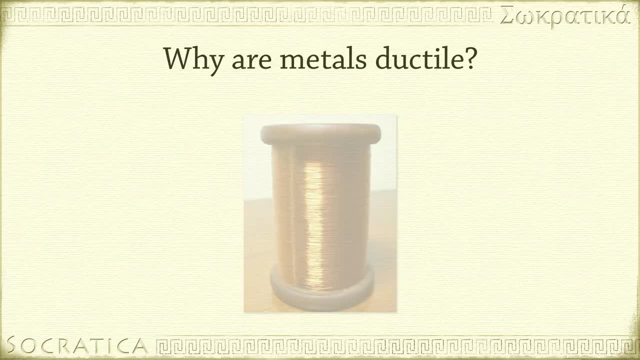 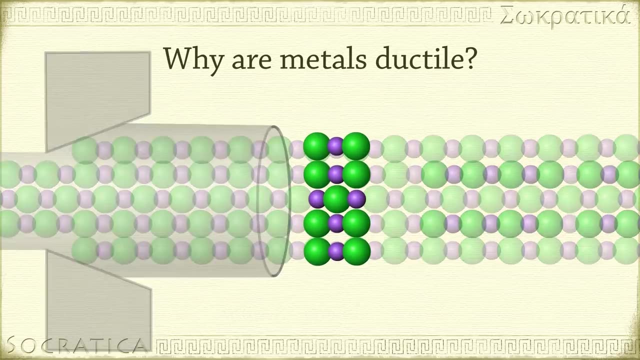 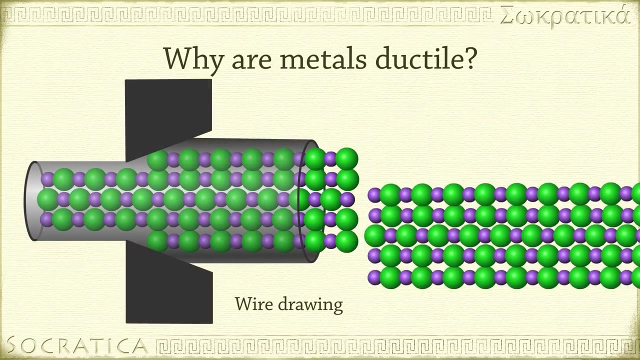 thin wires. We call this ductility. Ionic compounds are not ductile. for the same reason, they are not malleable in general. If an ionic compound is forced into a long cylinder, it breaks apart because of the repulsion of like ions In. 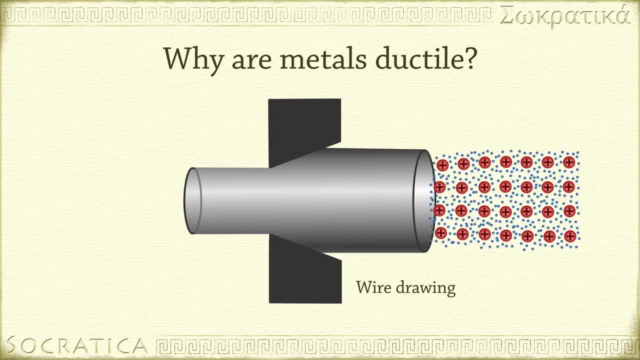 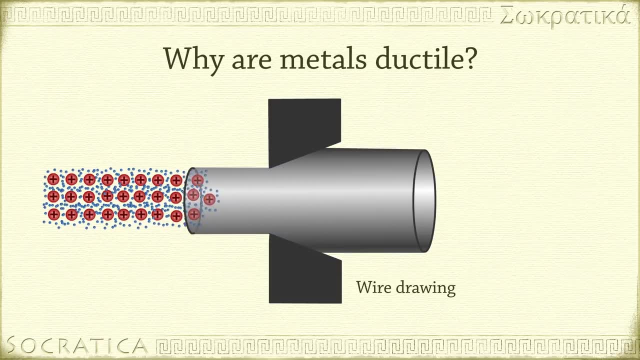 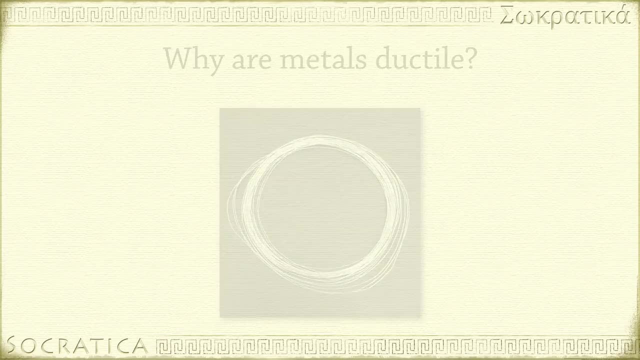 contrast, a metal can be pulled into a long cylindrical shape because the cations can line up, shielded from each other, as the fluid-like sea of electrons flows around them. The most ductile metal is platinum. Almost all metals are solid at room temperature, the cations forming a